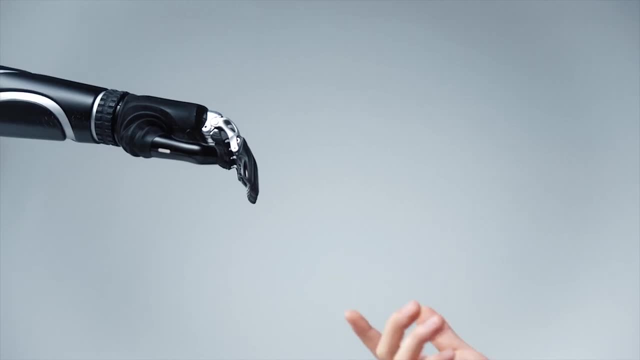 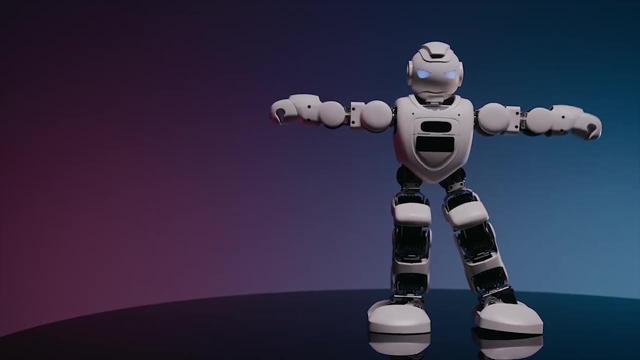 Thus, the functional end of a robot arm intended to make the effect, whether a hand or tool, are often referred to as end effectors, while the arm is referred to as a manipulator. Most robot arms have replaceable end effectors, each allowing them to perform some small range. 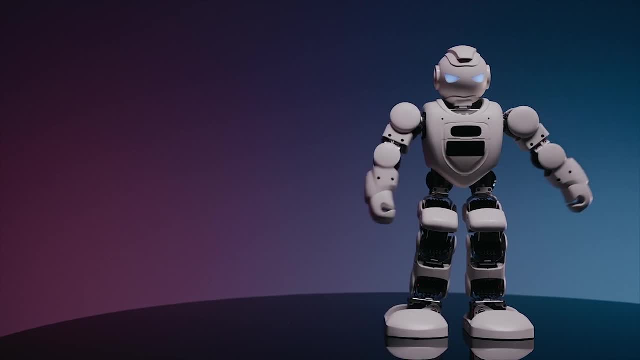 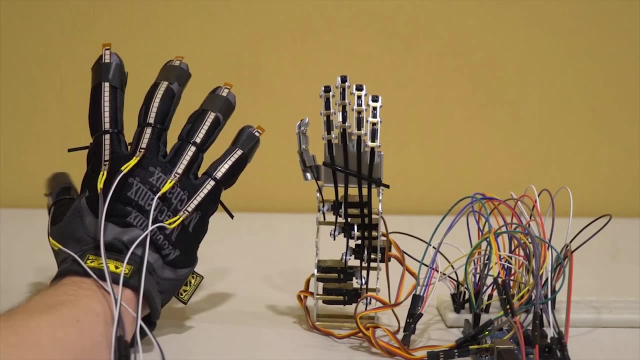 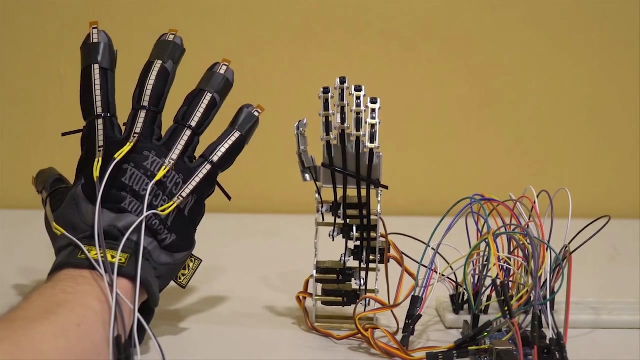 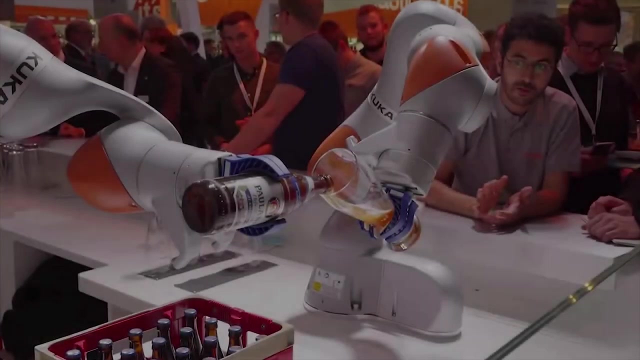 of tasks. Some have a fixed manipulator that cannot be replaced, while a few have one very general purpose manipulator, for example, a humanoid hand. What is robots manipulator? In robotics, a manipulator is a device used to manipulate materials without direct physical contact by 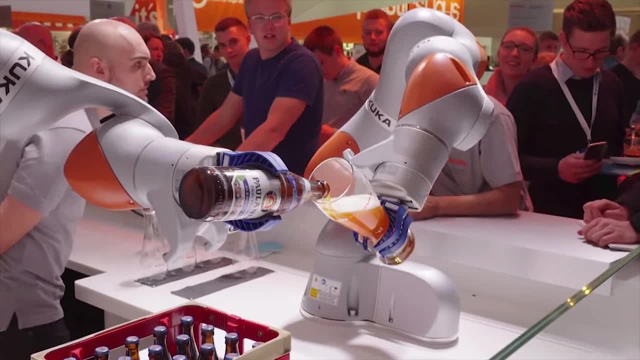 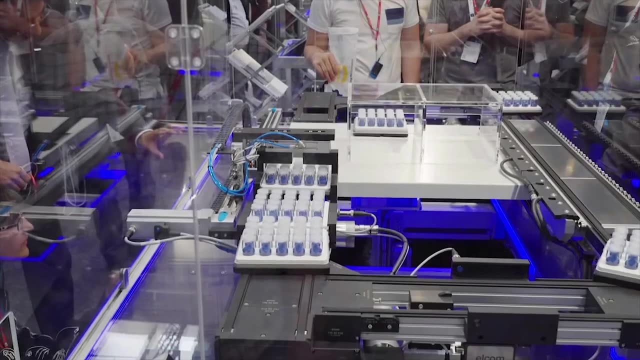 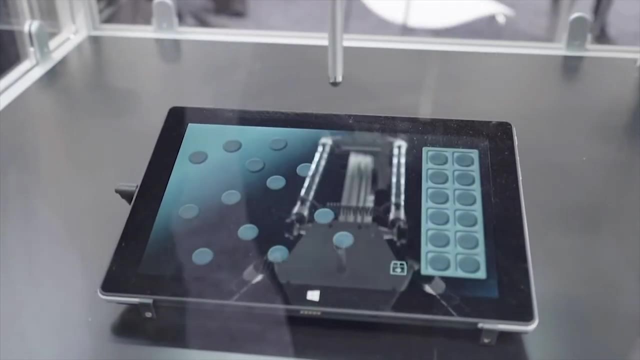 the operator. The applications were originally for dealing with radioactive or biohazardous materials using robotic arms, or they were used in inaccessible places. In more recent developments, they have been used in diverse range of applications, including welding, automation, robotic surgery and in space. It is an arm-like mechanism that consists of a series of segments. 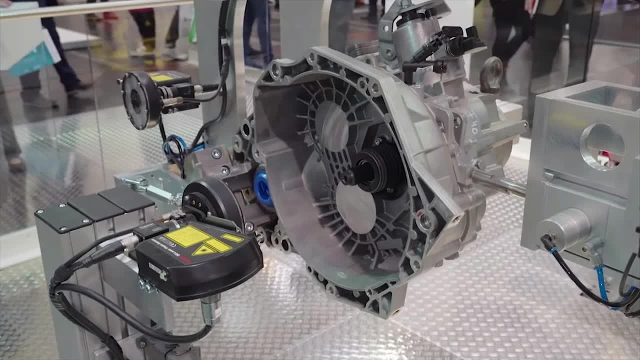 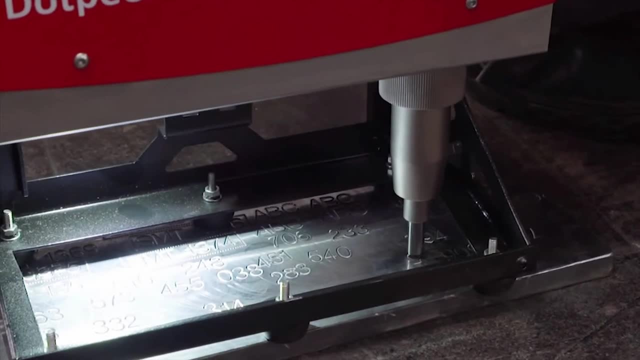 usually sliding or jointed, called cross slides, which grasp and move objects with a number of degrees of freedom. In industrial ergonomics, a manipulator is a lift assist device used to help workers lift, maneuver and place articles in process that are too heavy. 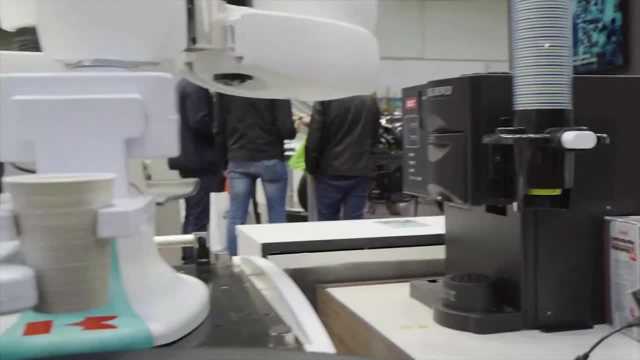 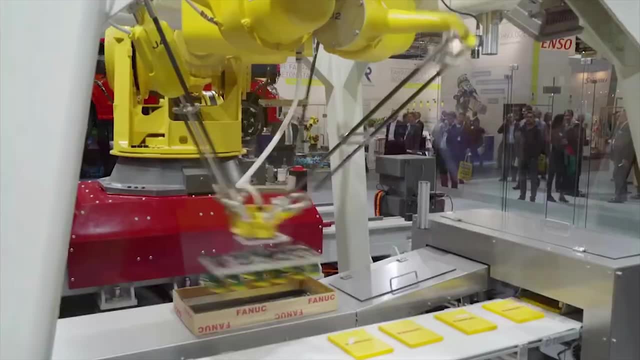 too hot, too large or otherwise too difficult for a single worker to manually handle, As opposed to simply vertical lift assists, cranes, hoists, etc. manipulators have the ability to reach into tight spaces and remove workpieces. A good example would be removing 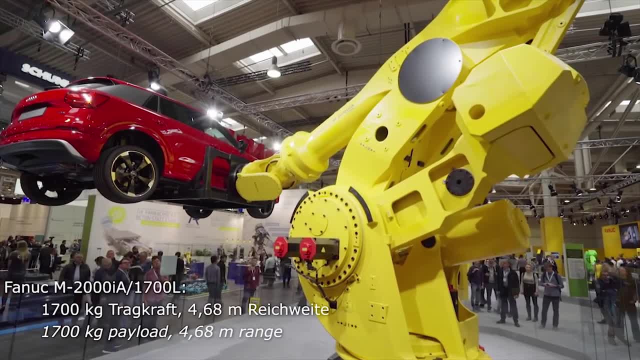 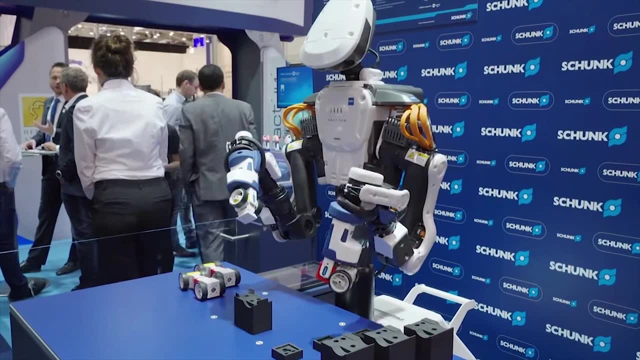 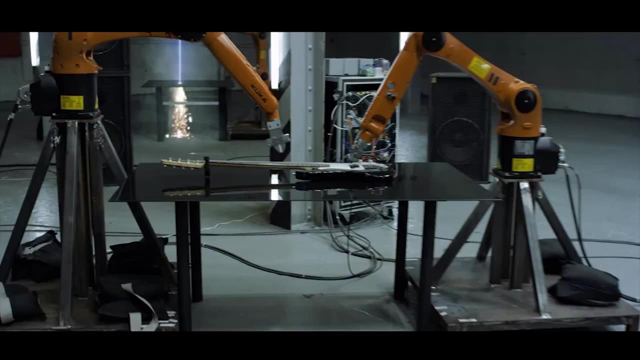 large stamped parts from a press and placing them in a rack or similar dunnage. In welding a column, boom manipulator is used to increase deposition rates, reduce human error and other costs in a manufacturing setting. Additionally, manipulator tooling gives the lift assist the ability to pitch, roll or spin the part for. 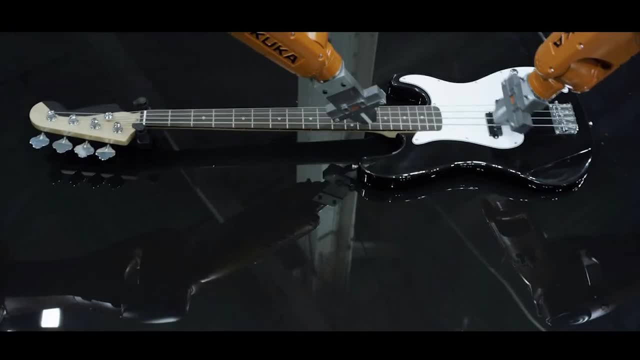 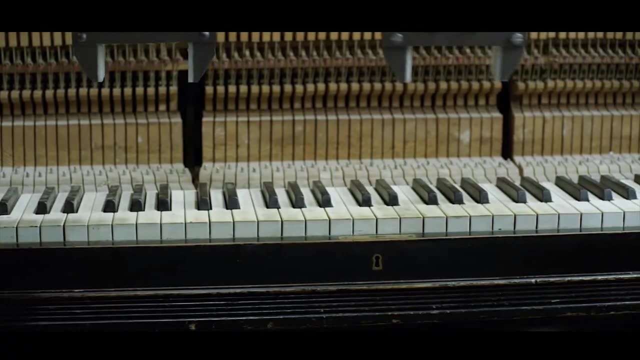 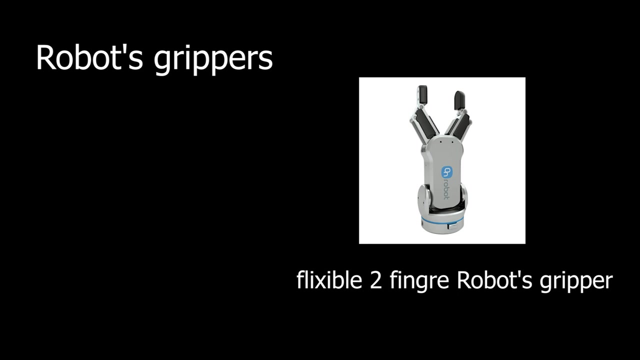 appropriate placement. An example would be removing a part from a press in the horizontal and then pitching it up for vertical placement in a rack, or rolling a part over for exposing the back of the part. What are robots? grippers? Grasping is force closure. Generally, the gripping mechanism is done by the grippers. 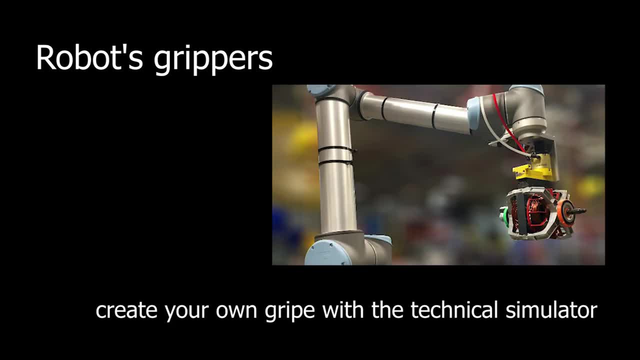 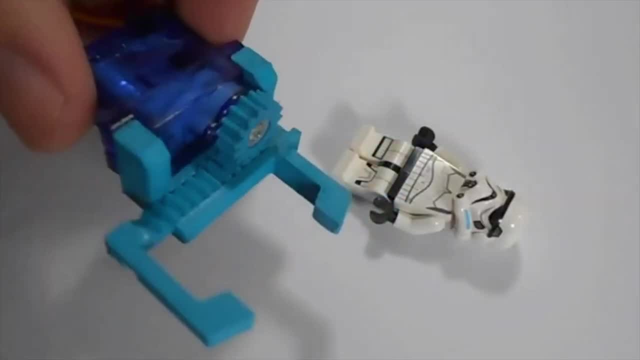 or mechanical fingers. Two-finger grippers tend to be used for industrial robots performing specific tasks. in less complex applications, The fingers are replaceable. Two types of mechanisms used in two-finger gripping account for the shape of the surface to be gripped. 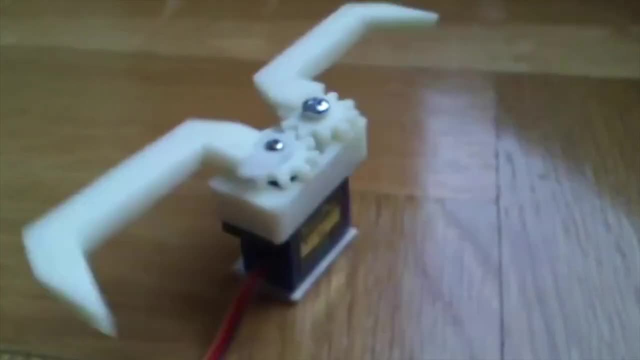 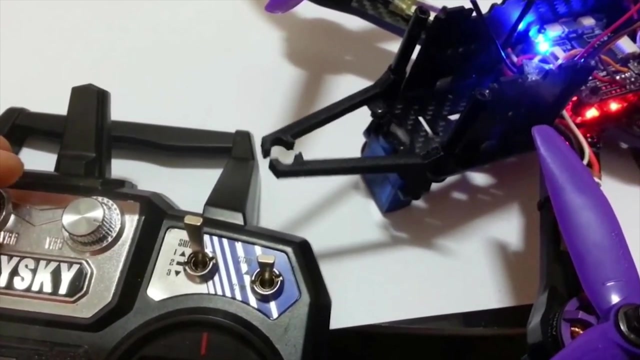 and the force required to grip the object. The shape of the finger's gripping surface can be chosen according to the shape of the objects to be manipulated. For example, if a body is designed to lift a round object, the Kripper surface shape can be a concave impression. 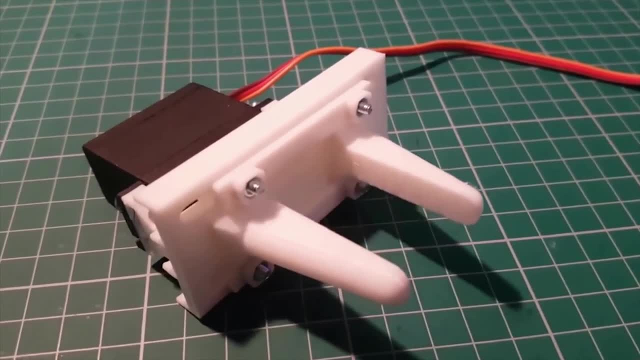 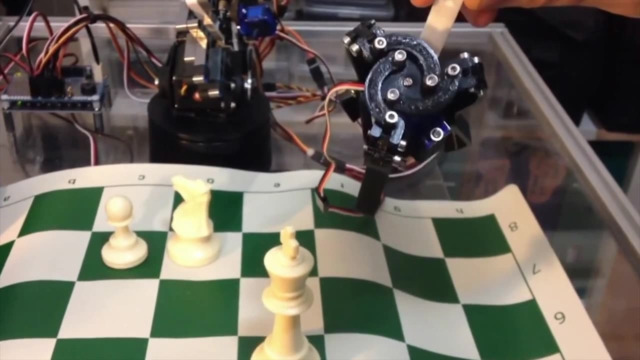 of it to make the grip efficient. For a square shape, the surface can be a plane. Though there are numerous forces acting over the body that has been lifted by a robotic arm, the main force is the frictional force. The gripping surface can be made of a soft material with. 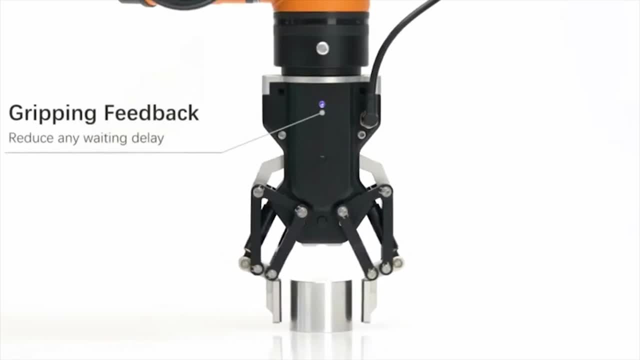 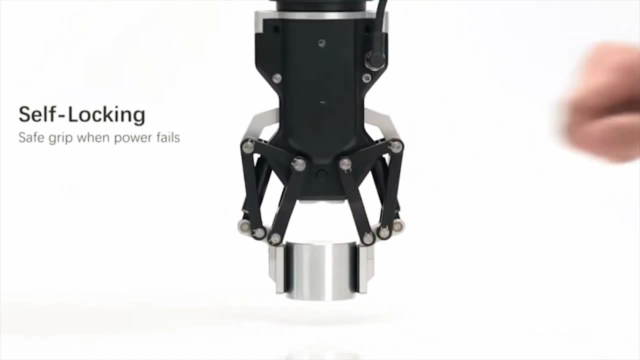 high coefficient of friction so that the surface of the object is not damaged. The robotic gripper must withstand not only the weight of the object but also acceleration and the motion that is caused by this force, That is, any pressurecus, corner or small of a. 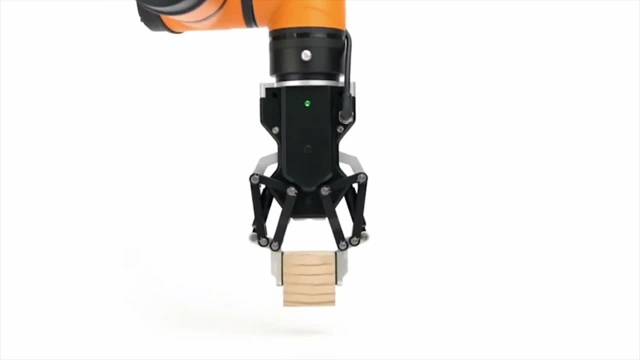 single ball in solidключed hands, The masse gremos, each of the force Station of friction, VRG facilities, even the final performance of the architecture: Volume, the, its size and the by frequent movement of the object To find out the force required to grip the object. 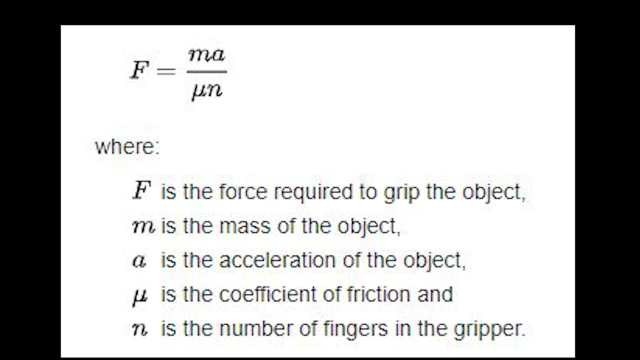 the following formula is used: F equals m a by q. n. Were F equals the force requires the object. M equals is the mass of the object. A equals is the accelerator of the object. Q equals is the co-effect of the fraction. N equals is the number of fingers in the gripper. A more complete equation. 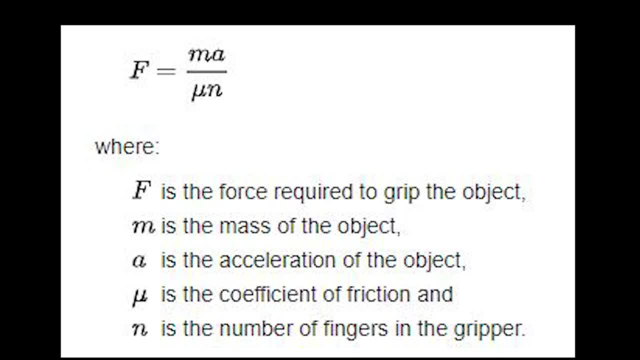 would account for the direction of movement. For example, when the body is moved upwards against gravitational force, the force required will be more than that towards the gravitational force. Hence another term is introduced and the formula becomes: F equals m, a plus g by q, n Here. 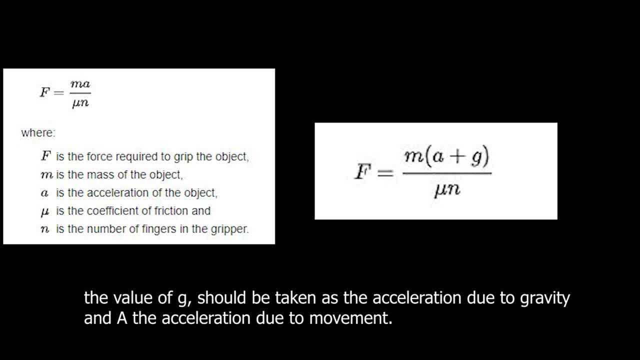 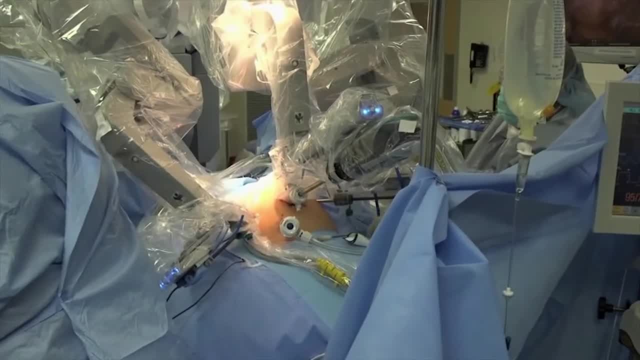 the value of g should be taken as the acceleration due to gravity and a the acceleration due to movement. What is robotics tweezer? Tweezers are small tools used for picking up objects too small to be easily handled with the human fingers. The tool is most likely derived from tongs.